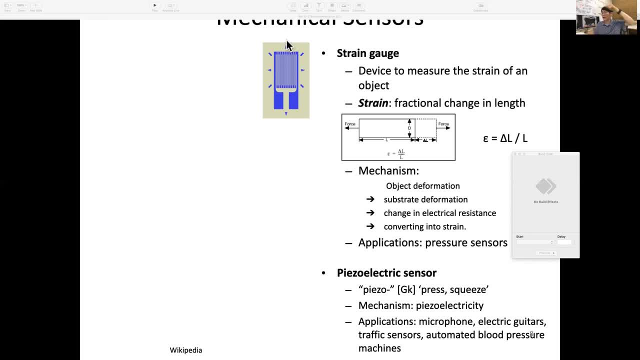 case, measures. this ups and downs the strains, And deformation of this object gives a substrate deformation and that results in changes in electrical resistance And you can convert that resistance change into the strain. So let me give you an example: Pressure sensors. So you like music and guitar. 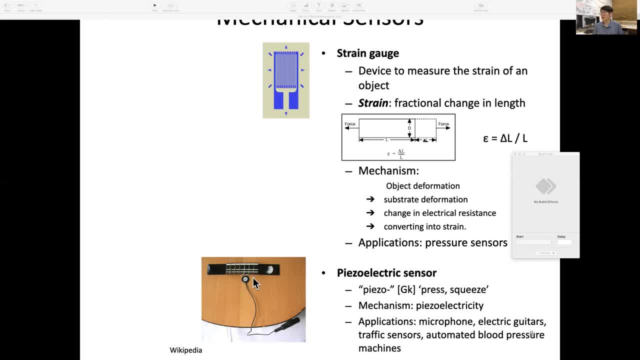 like electric guitar. This piezoelectric- not piezo, It's a strain gauge. It's used here to detect and amplify and converting this sound into an electrical signal, And the mechanism is pretty simple. It's a kind of like a metal detector, So it's a 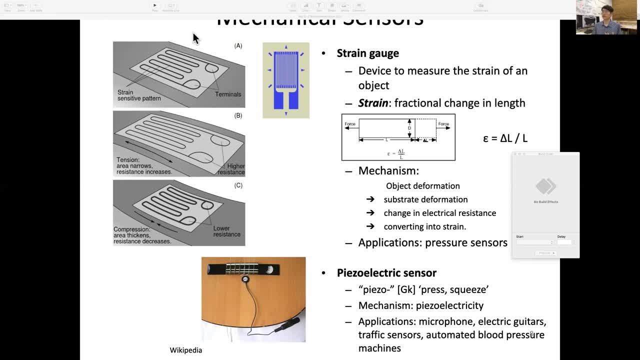 pretty simple. you see these actual ones into a cartoon, then strain sensitive pattern. in this case you see this directional change. so that's more like this directional strain we are measuring. so when there's a, let's say, tension, then it elongates. 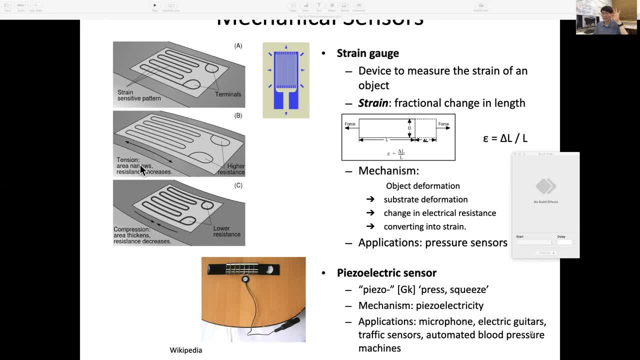 so then the cross-sectional area narrows down. that means electrical resistance goes up, While compression case, that area becomes thickened, and so the resistance will go down. So this very simple principle is being used for measuring strain, and that can be measured for. 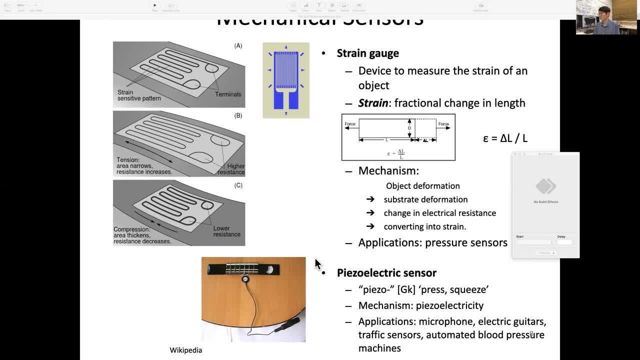 in this case the pressure changes. So piezoelectric sensor is another. that piezo means press and squeeze, which will generate piezoelectricity. So microphones, electric gears, guitar, traffic sensor, even automated blood pressure machines uses piezo. 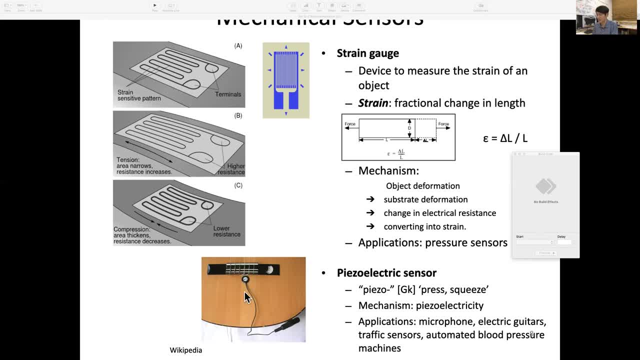 Sorry, I have to correct it. this guitar ones are actually piezoelectric sensor which measures this pressure and directly convert into the voltage, And so that is a piezo. you see, this pressure, mechanical pressure, can induce a voltage change. 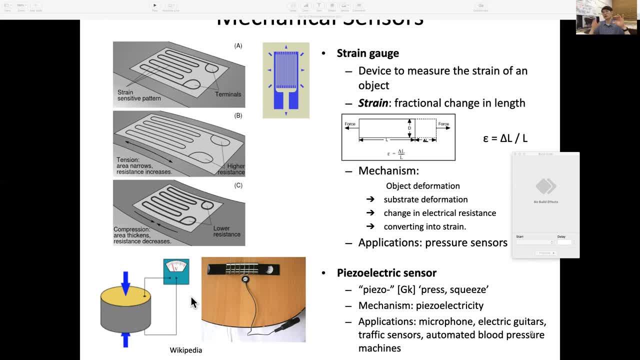 In fact, this piezo can be used in reverse, which means you give a voltage to apply to piezo and the piezo will deform. In fact, my PhD thesis. I use a piezo, a linear piezo. I give certain voltage to make a piezo to displace.